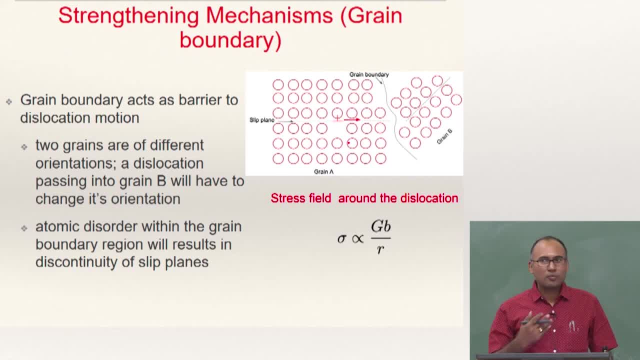 nano crystalline materials. so, for instance, nano crystalline copper and a coarse grained copper, So polycrystalline copper, which is coarse grained. it is a material that is not. This is a nanocrystalline copper. If you take these two materials, both of them will not give you same strength because of 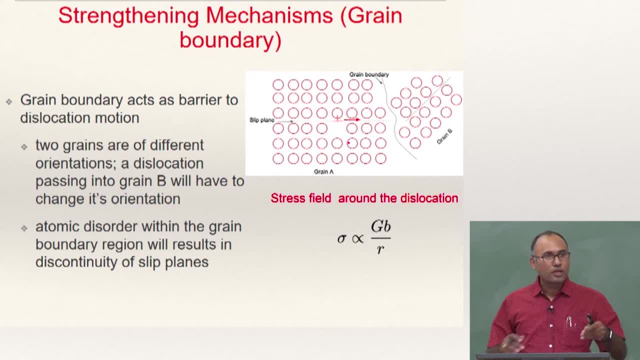 the fact that the grain size is smaller. in nanocrystalline material you have more grain boundary area and hence there is a higher probability for the dislocations to go and get pinned near the grain boundary, and hence nanocrystalline materials are stronger and 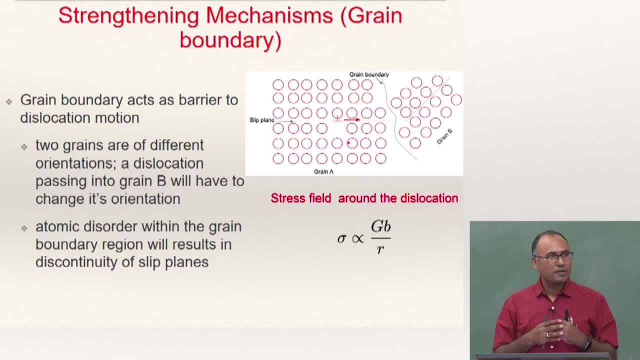 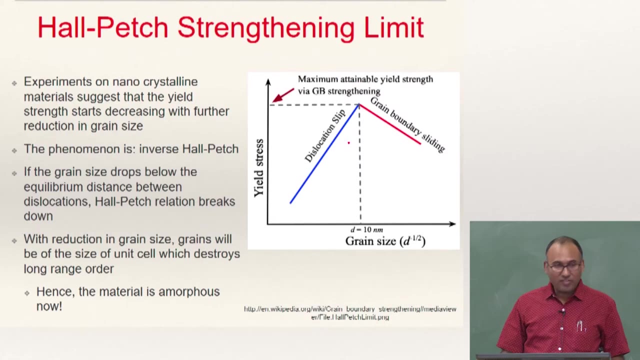 in other words, people usually call this phenomena as smaller is stronger, so you should not look down upon small things, right? smaller is harder and stronger. that is very important to, even in material science. okay, And then we have also discussed about halpedge, that is, as you reduce the grain size. this 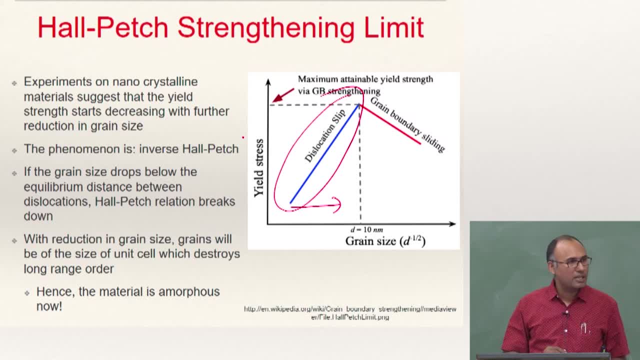 is the reduction in size of the grain. you are increasing the yield strength of the material, but there is a size about which this halpedge can be reduced. This halpedge relation breaks down and beyond if you further reduce the grain size again. 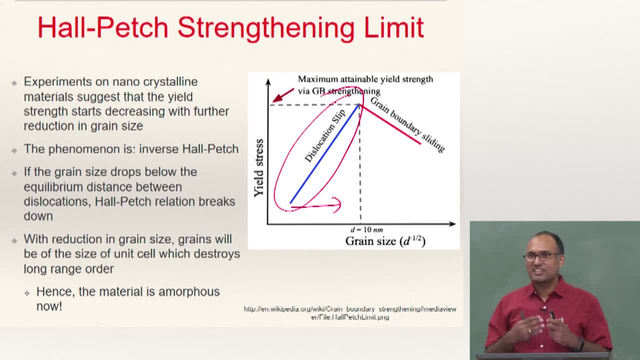 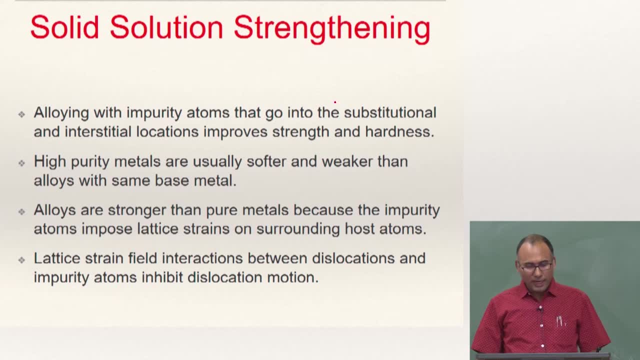 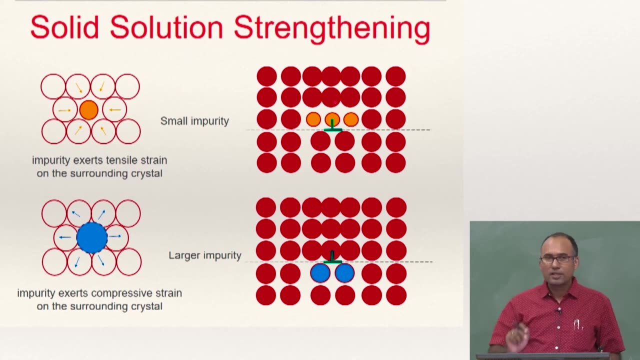 the yield strength starts to decrease. okay, we have discussed that as an inverse halpedge relation and we have also discussed why that is so okay. And then we have discussed about solid solution strengthening. so when you put in an impurity element, then actually that locally changes the stress state and the dislocations have. 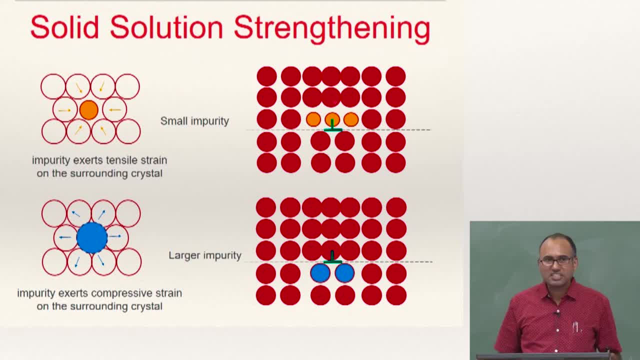 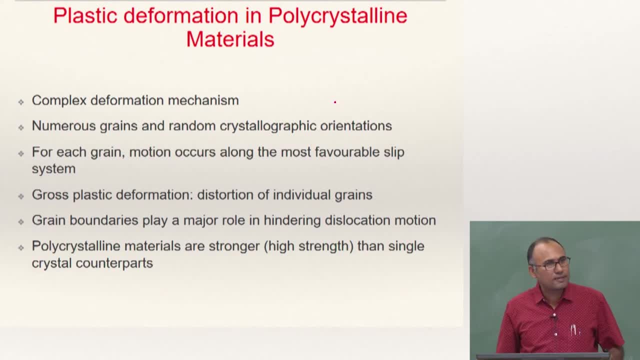 to interact with the stress state. as a result, your material gets strengthened, And we have also. I have not written here, but we have also discussed the strain hardening or work hardening, both in single crystal material as well as polycrystalline material. 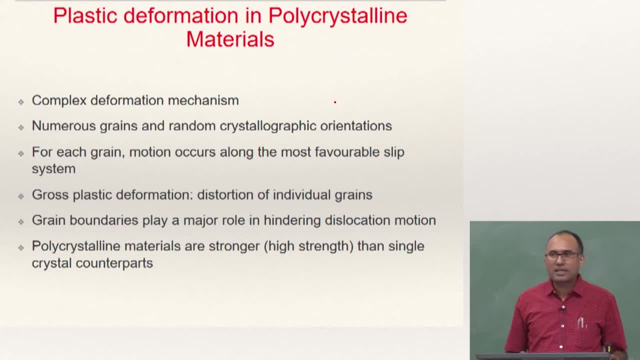 In the single crystal material it is typically the stage 2, wherein when you increase the dislocation density, these dislocations start interacting with each other. so dislocation entanglement might happen. dislocation, annihilation may happen, dislocation- you know the dislocation. 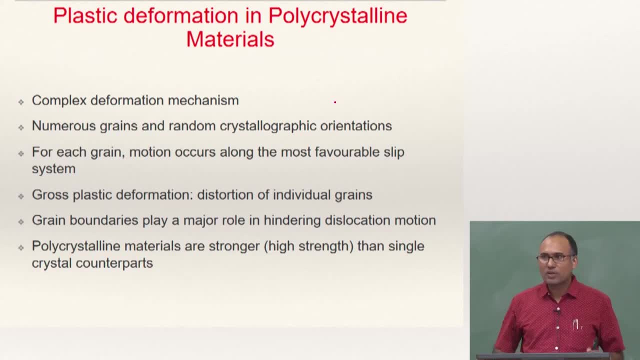 repulsion may happen. all these interactions will actually impede dislocation motion and the strengthening is nothing. but we have just now we have actually defined the process of strengthening as a way of impeding the dislocations. right, If we impede the dislocation motion, that will enhance the strength of the material. so all 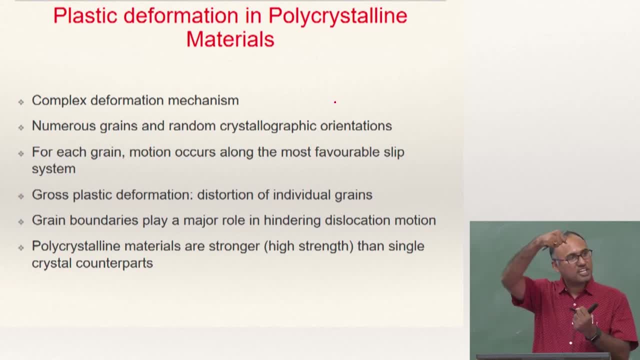 these things impede. so that is why, as you continue to increase the strain in the material, there are dislocation, density increases, Okay- And they start to interact and, as a result, you are going to have more and more strength for the material. 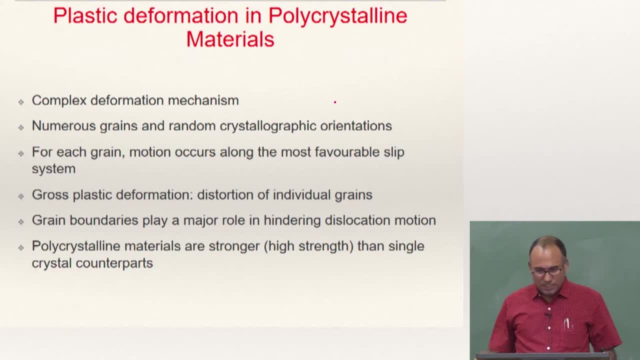 Okay, Alright, Now we will look at plastic deformation in polycrystalline materials. In polycrystalline materials it is a little bit more complex than a single crystal material, because in single crystal material you, first of all, you do not have grain boundaries and 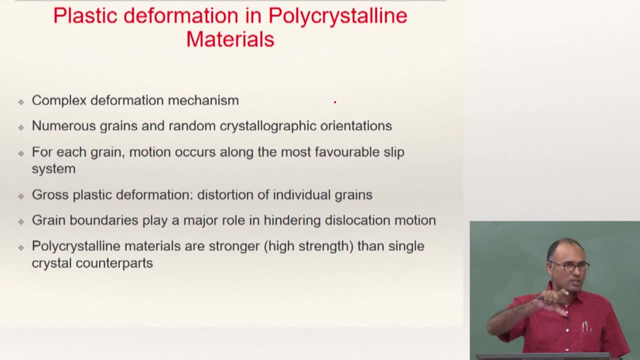 the second thing is that you have slip systems in a particular grain and then those slip systems may interact, But in a polycrystalline material- the slip system, you can have slip, initial slip, getting activated on several grains, because you have one slip in a single crystal material. you 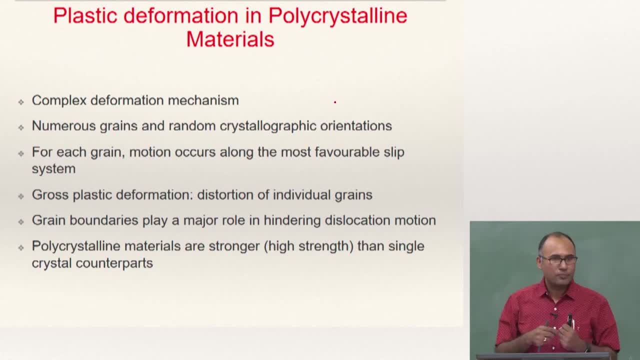 have one slip system that is favorably oriented typically, but the fact that you have a polycrystalline material, it is possible or it is probable that there are more number of slip systems active to begin with And, as a result, it is not possible. 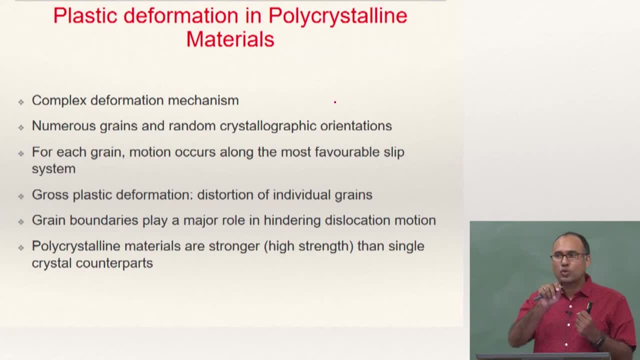 Okay, Okay, Okay, Okay. So it is not possible for you to observe this easy glide so easily in a polycrystalline material. Okay, So, easy glide is not something that is usually observed in polycrystalline material. 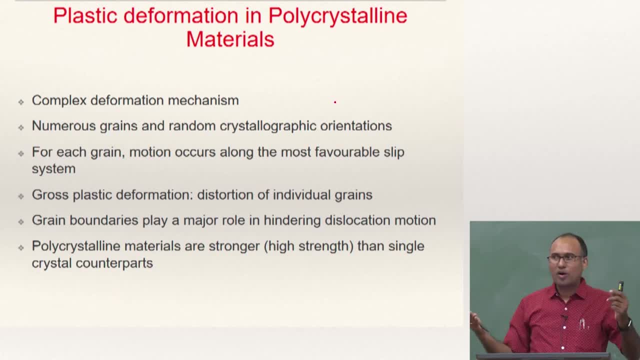 You will have a yield strength and immediately your strain hardening starts because several dislocations in several slip systems or several grains start activating and they start interacting with the grain boundaries and so on. Okay, So hardening kicks in quite early in a polycrystalline material and you should be able to see why. 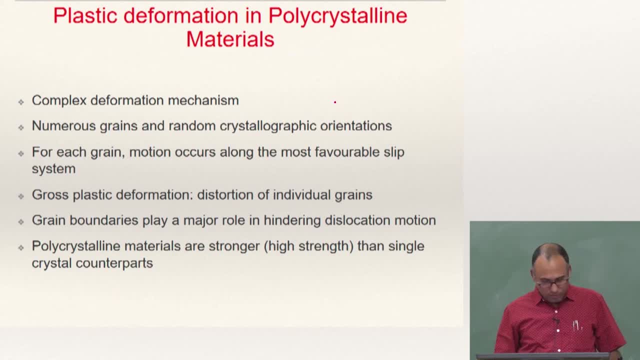 it does so Okay, And as a result, we have also discussed that the polycrystalline materials are stronger than their single crystal components. So if you make a single crystal copper and a polycrystalline copper, single crystal copper, 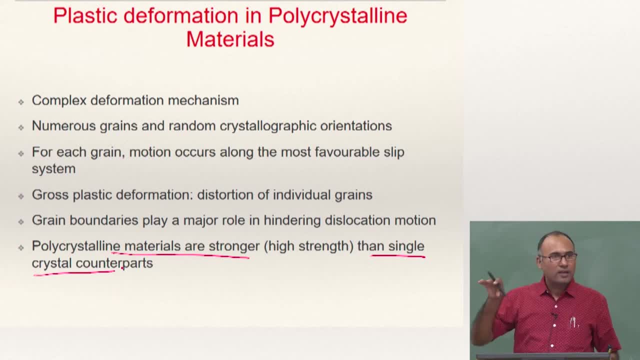 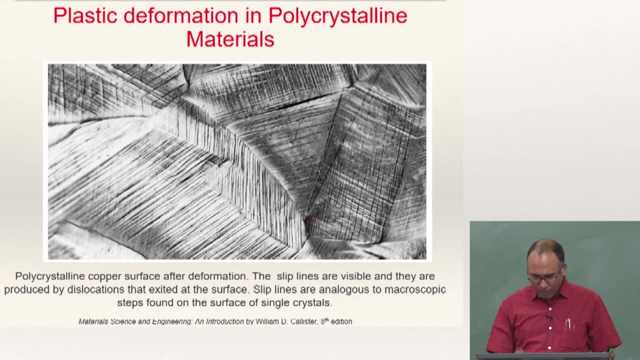 is going to be softer compared to polycrystalline copper because of the impediment of dislocations in a polycrystalline material compared to a single crystal. plastic deformation on a polycrystalline material. So these are your slip lines. you will see in a single crystal, in a single grain, you 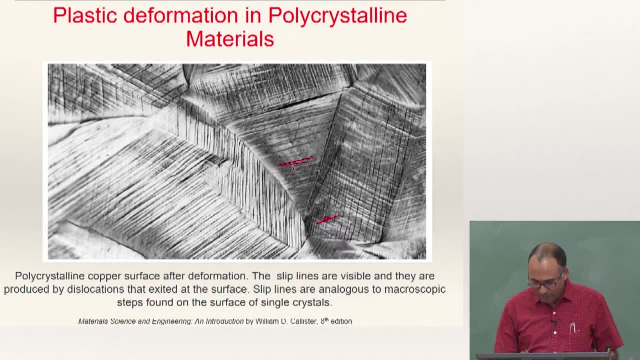 have several slip systems activate active right. Some of these things are one slip system and there are other lines like that. so that means in one grain more than one slip system is active. that is one thing, and there are several grains in which several slip systems are active right. 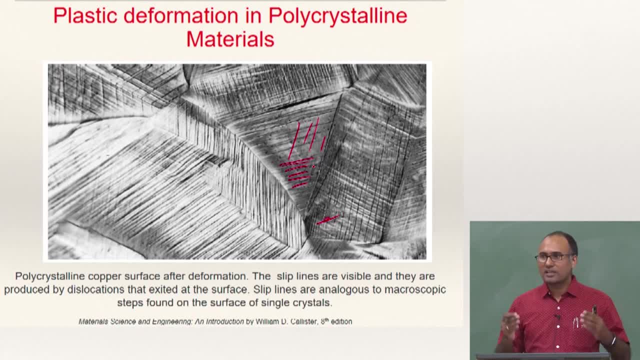 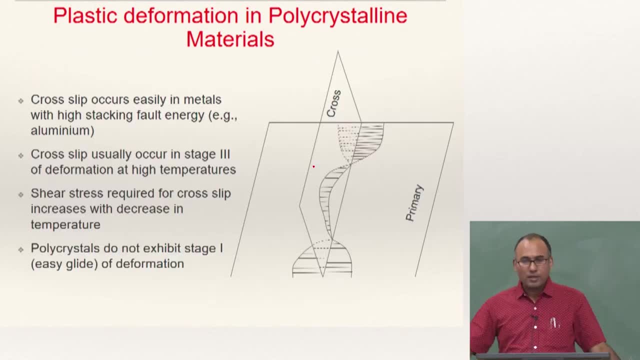 So all these things can actually be working in concert in a polycrystalline material. That is, your slip system 1, slip system 2, and so on. The another mechanism that is important in a polycrystalline material is something called 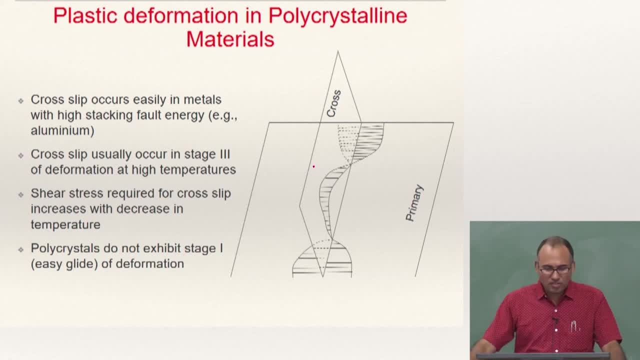 cross slip. So what do you mean by cross slip? So it typically occurs in stage 3 of deformation at high temperature. So this is your one slip system and this is another slip system. So then the dislocation might actually jump from one guy to another. 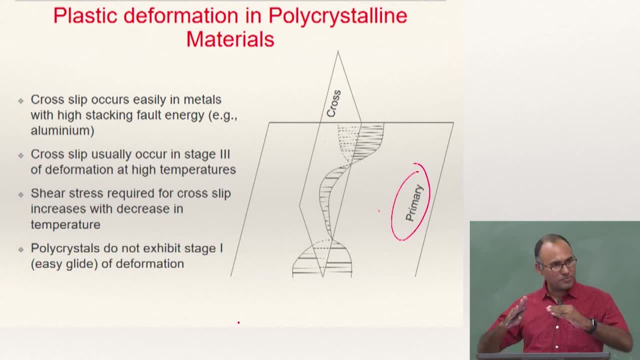 So there can be a slip happening from one slip system to another slip system, and this is what we call cross slip And, as we have already discussed, the polycrystals do not exhibit stage 1 of deformation. That is very difficult to observe stage 1 of deformation in polycrystalline materials. 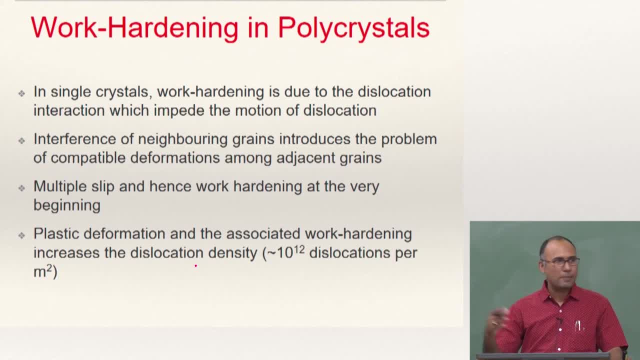 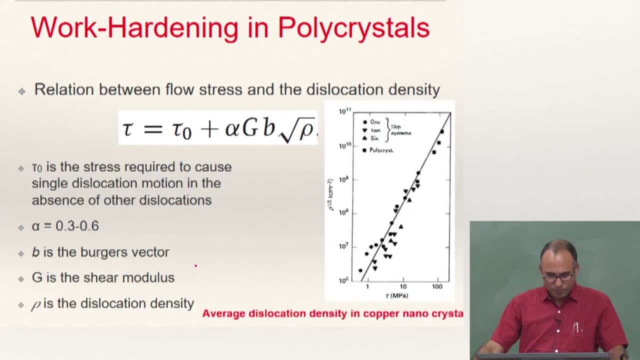 And we have also discussed about work hardening because of the multiple slip and there is going to be more resistance for the dislocation motion And the relation between shear stress and the dislocation density. so this rho is your dislocation density right. 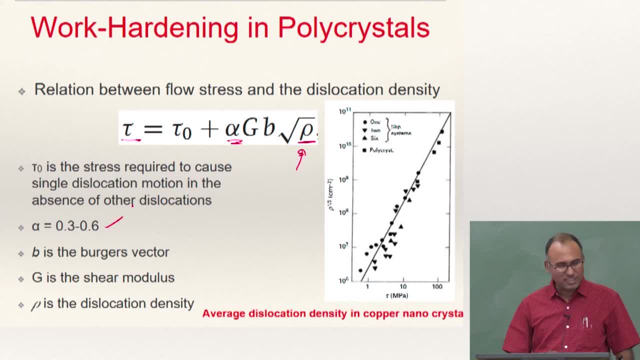 And alpha is a material parameter. Typically for metals it is between 0.3 and 0.6, and g is your shear modulus, b is your Burgess vector, And then, as you continue to load the system, your dislocation density increases, right. 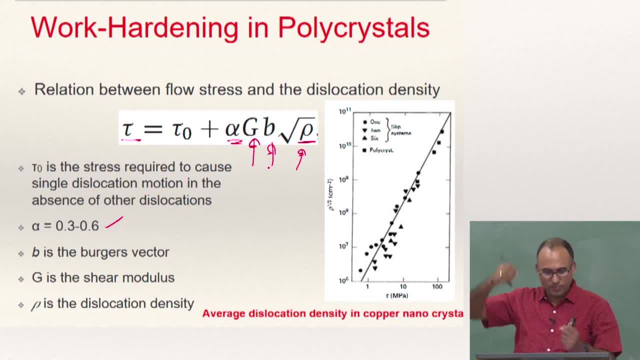 Because the number of dislocations are multiplying as you continue to load the system. So, because of the fact that the dislocation density is increasing, your shear stress required to cause further deformation increases. And that is how the dislocation density and flow stress in a material are connected. alright, 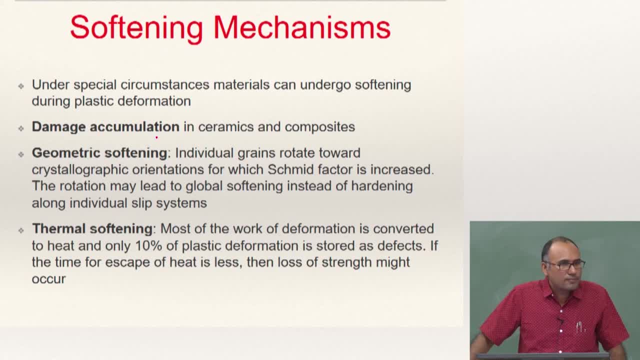 So far we have discussed about hardening mechanisms. but in materials it is also possible that there are certain mechanisms which makes the material soft right, So under special circumstances they can undergo softening. during plastic deformation That happens when you have damage. So what do you mean by hardening? 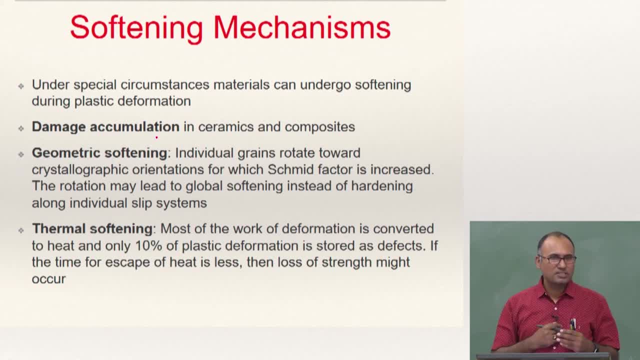 The material is becoming more and more stiffer, right, Is not it? If you see your strain response, your elastic stiffness, and then it is becoming to cause same strain, you are actually requiring to apply more hardening Stress. right, It is becoming harder. 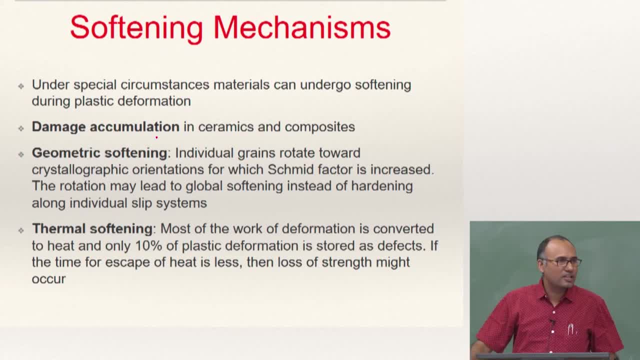 But if you have a damage in the material, that means during the deformation you are imparting damage to the material and that damage actually is going to reduce the overall elastic stiffness of the material And that is what you mean by softening that. So damage accumulation is one of the mechanisms. 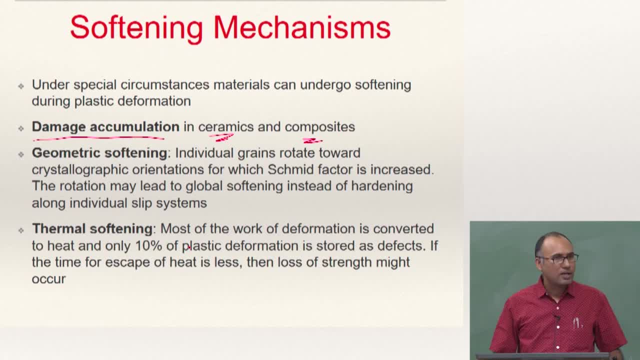 This is typically observed in ceramics and composites and ceramics. you can clearly see that there is no plastic deformation, right. So the plastics fail by damage accumulation, that they typically fail by brittle impact. And then there is another thing called geometric softening. What do you mean by geometric softening? 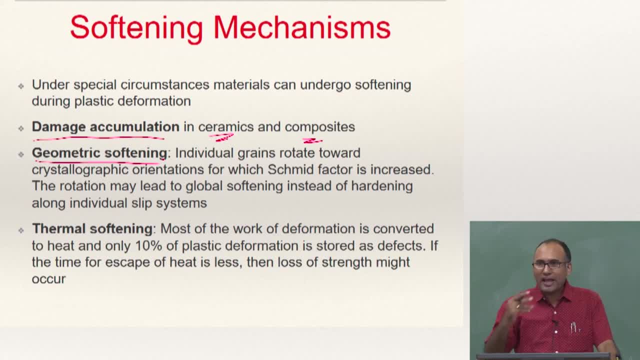 If it is softening, in other words, actually means that it becomes easier for you to impart dislocation. That is what you mean by softening. Hardening is becomes easier, difficult for you to impart dislocation. So hindering the dislocation motion is what causes hardening. 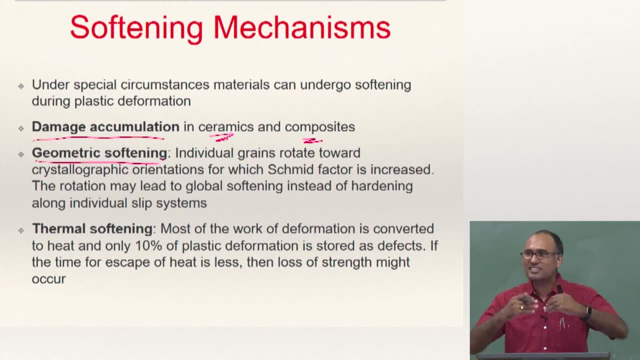 Okay, Thank you. Enhancing the dislocation motion is what causes softening. they are two opposing elements. So now, geometric softening means when you are applying a load, some of the slip systems are active right, And we also know that as you are deforming the material, the slip system orientations 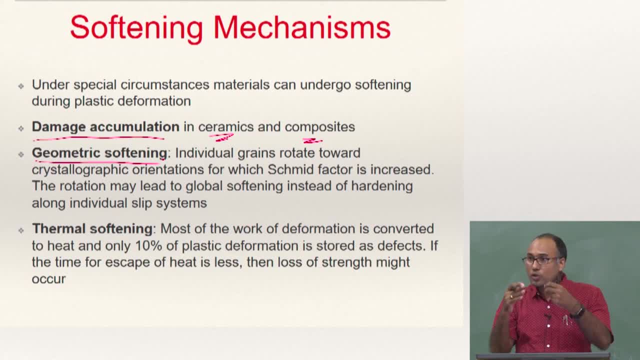 are changing, the slip systems will be rotating And during this process it is possible that there are more and more slip systems that are changing their orientations in such a way that you are enhancing the dislocation motion. That means there are more slip systems that are becoming favourable or active, because 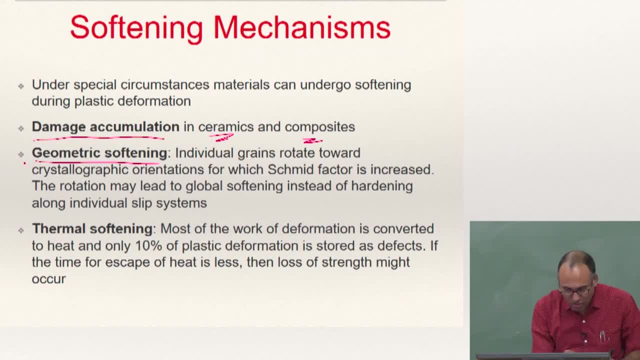 of the geometric orientation changes and that such a softening mechanism is called geometric softening. okay, So the individual grains rotate towards crystallographic orientations for which Smith factor is increased. When your Smith factor is increased, then it becomes easier for you to cause plastic. 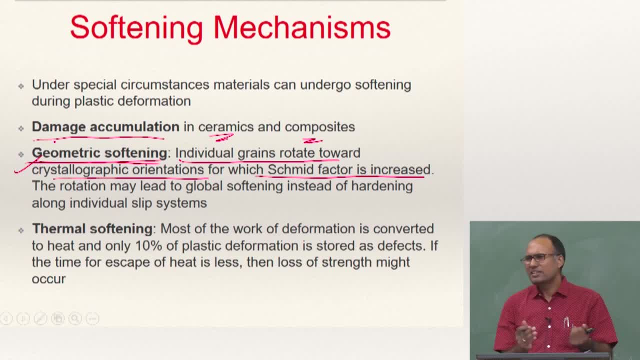 locomotion or dislocations, And that is what is happening. What is geometric softening? This typically happens in several materials, but many a times what happens is your hardening effect is more predominant compared to the geometric softening. Even during the hardening response, the crystal orientations are changing. 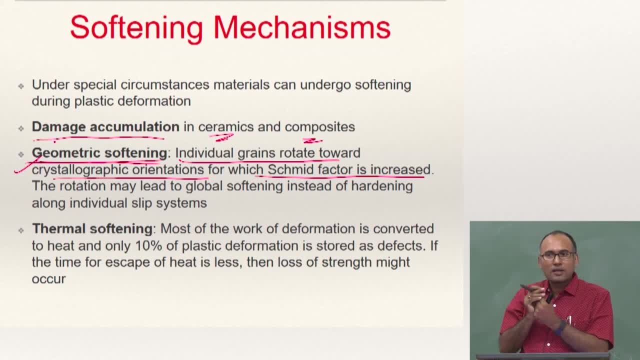 But the effect caused by reorientation of the crystals, the grains, is actually much less compared to the effect caused by the dislocation, the obstacles in the dislocation. That is why, when you are seeing the hardening, you probably would not observe, you will not. 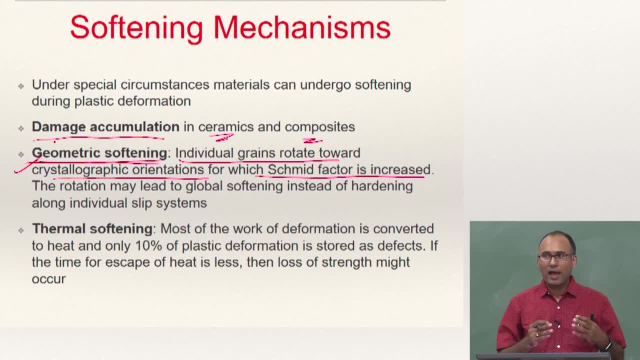 be able to observe softening, But in some situations you will have the several slip systems orienting in such a way that the Smith factor is actually going to be much higher. Then you will see a gross softening response of the material. And another way that you can impart softening is thermal softening. 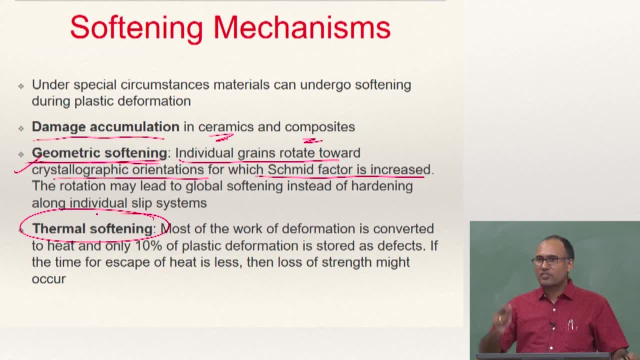 What do you mean by thermal softening? When you cause plastic locomotion, you will have a thermal softening. What do you mean by thermal softening? When you cause plastic locomotion, you will have a thermal softening. And when you cause plastic locomotion, you are actually creating, so there will be local. 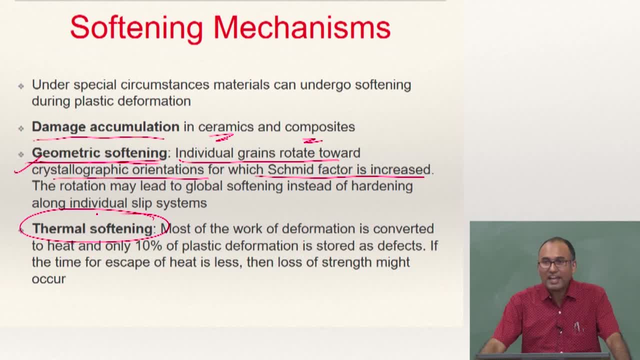 heat generation right, And the local heat generation might actually reduce the strength of the material And that is what we call thermal softening. So the heat generated because of the plastic deformation is what helps the enhancement of the dislocation. And these are the ways, different ways, that you can impart softening in a material. 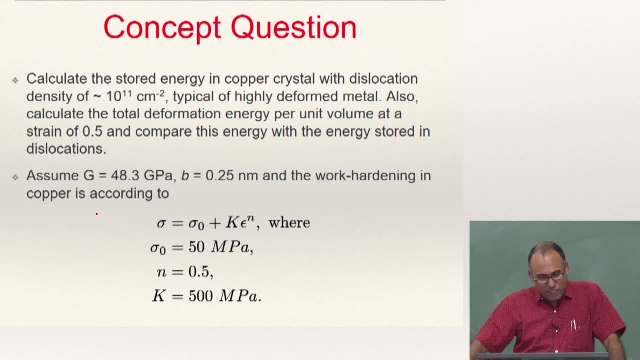 So now we are required to calculate the stored energy in copper crystal with dislocation density of 10 power, 11 per centigrade. So this is the dislocation density. This is typical of a highly deformed material. So this is actually highly deformed material. 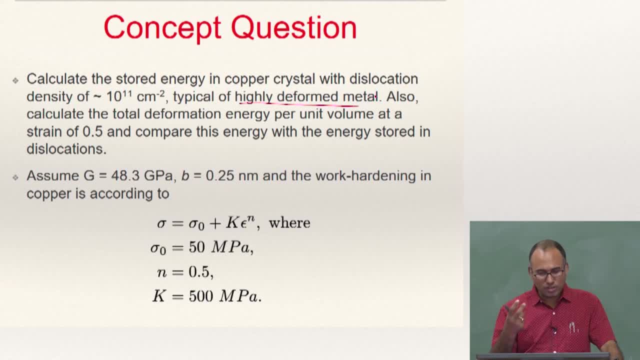 Also. so what we need to calculate? what is the energy, what is the total stored energy at the dislocation because of the presence of stress. So calculate the total deformation energy per unit volume at a strain of 0.5.. So if you are applying a strain of 0.5, what is the total deformation energy? and compare. 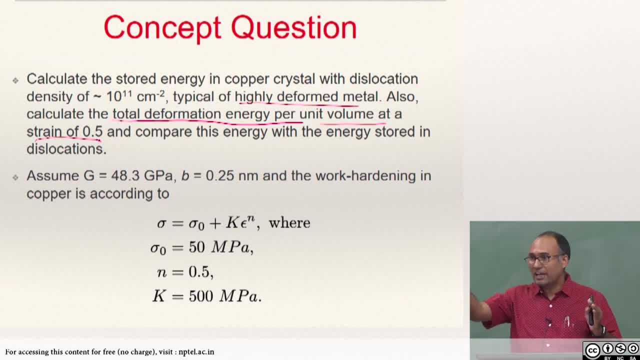 this total deformation energy with the energy stored in the dislocation. So you are taking a material, you are applying some load and then you are increasing the dislocation density. So there is an energy associated with the dislocation or not? What is that? 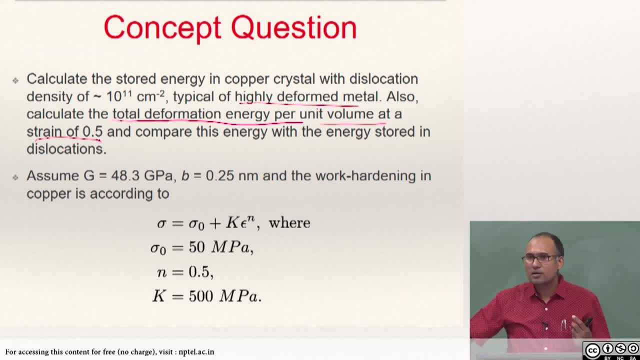 How do you calculate the energy associated with the dislocation Strain? energy associated with the dislocation is it depends on the burgus vector and shear modulus of G b square, that is the energy associated with the dislocation right. So now assume for this material the shear modulus is this: b is 0.25, that is burgus vector. 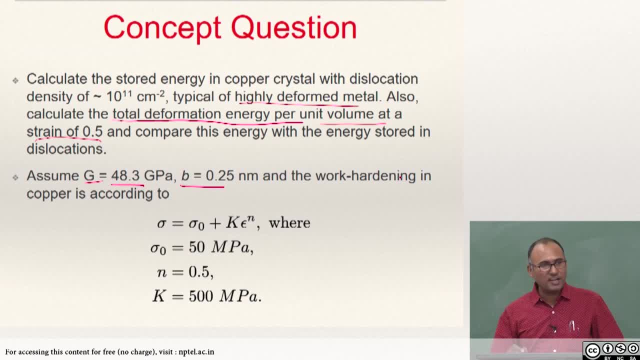 0.25 nanometer Right. What do you mean by work hardening? The hardening response during which the dislocation motion takes place is given by this formula: The sigma naught is 50 MPa. n is your hardening exponent. we will talk about this in a maybe. 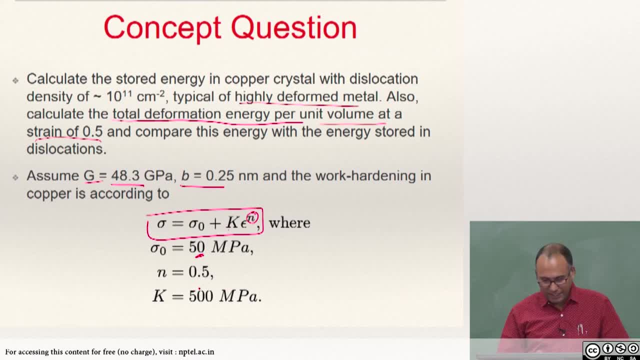 a couple of classes later. what is this? k and n? this is: this is a functional response of your stress flow: stress n equal to 0.5 and k is equal to 500 MPa. these are the material problems. 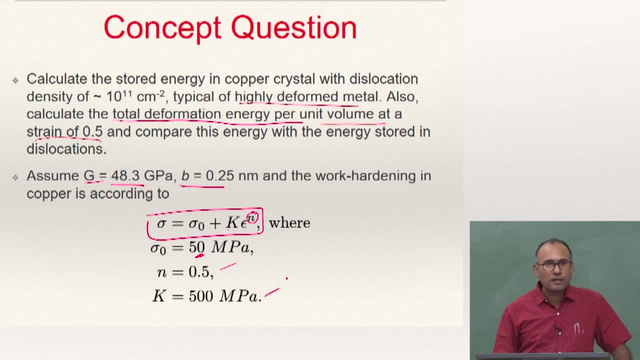 So if you want to, if you want to calculate the total deformation energy, you need to find out integral sigma times epsilon dv. that is your total deformation energy. you know what is your sigma and epsilon is going from 0 to 0.5 and that is your total right. 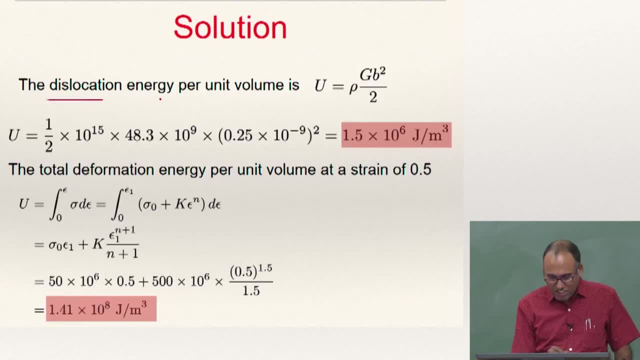 So let us try to solve this problem. So the total dislocation energy per unit volume is half rho gb square, and this rho is your dislocation density. g is your shear modulus, b is your shear modulus. So this is your total deformation energy. 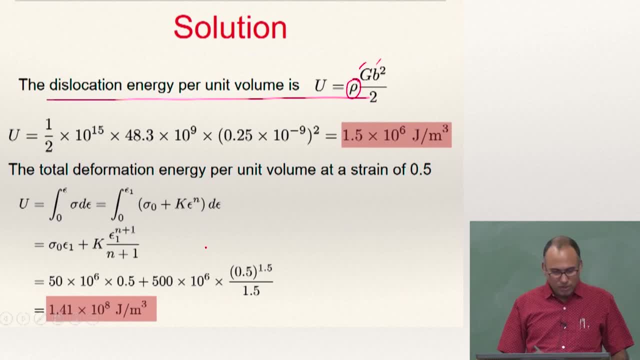 So this is your total deformation energy. So sorry, I should not have spoke so much to you, Because what we are discussing, we are gonna discuss about what is the type of obstruction of the material. also, in sequence related from the previous treatises, is that the construction. 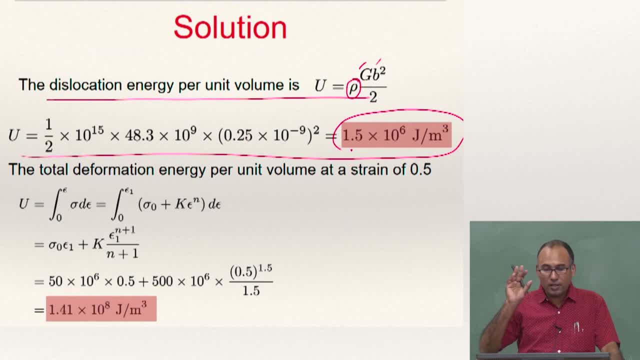 basis is the πάь ßb, so it is more or less same. taken funded matter, which has sometimes been considered part phi of energy, so необход dedicate gifted matter to surface of the material projectile. Okay, Now in the case of грnanitegers, for it is input theta equal to 1.2 and it is equal. 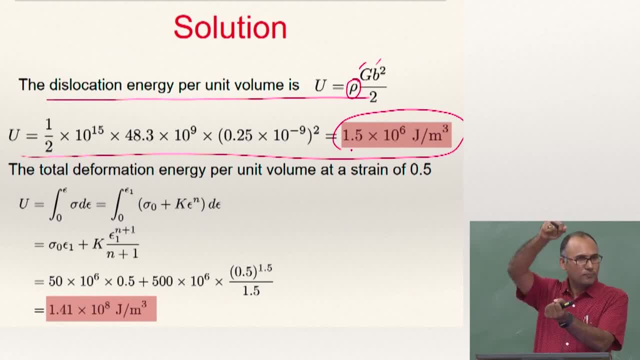 to 1, with deleted matter equal to 1, with votes alpha is equal to 2 and its geçal of theta equal to 1, and its going toy is 0x4.. This will be your principal in sequence right given by this expression, right? So the strain energy in material, in the material, is actually 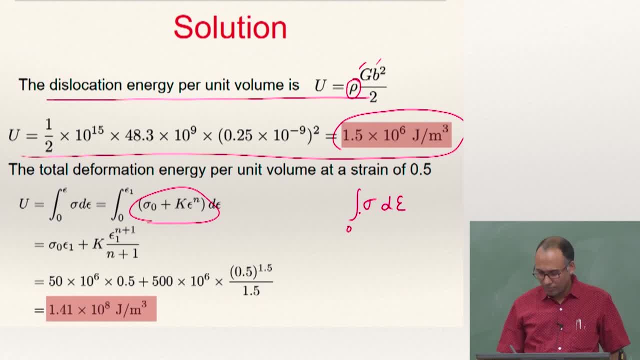 integral, sigma d, epsilon, going from 0 to epsilon. So you have no, you know what is your sigma and you know to which strain you have actually deformed the material and you calculate this integral, evaluate this integral. then you get 1.41 into 10 power 8, that means 140 megajoule. 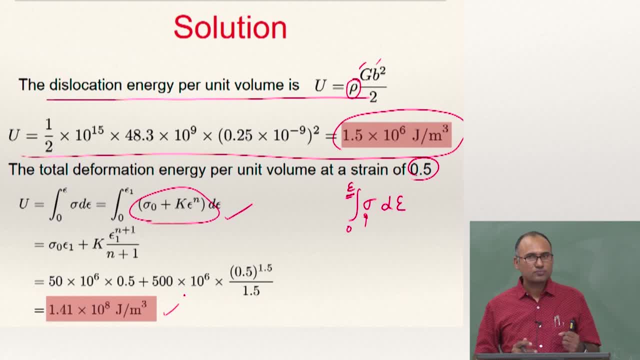 per meter cube. What is the meaning of this? You have deformed a material and to deform this material to a strain of 0.5, you have put in 140 megajoules per meter cube of energy. that is the total deformation energy. 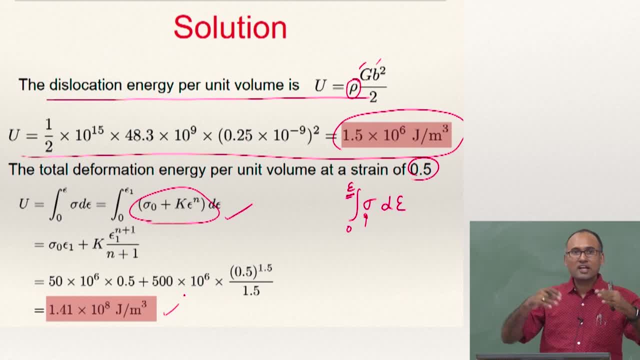 Now, when you have done this, there is there are some dislocations that are multiplying in the material. So you have got a final dislocation density of 10, power 11 plus n mu square, and the strain energy associated with those dislocations is calculated to be: